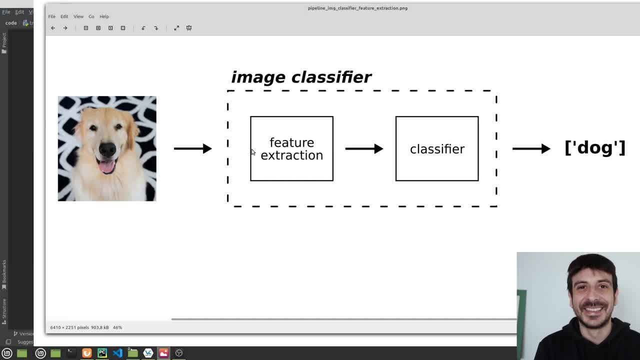 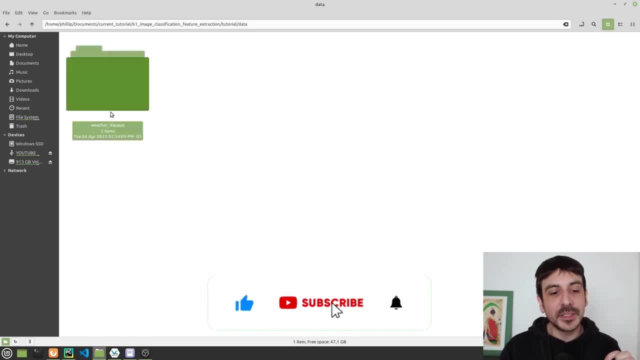 vision tutorial. and now let's get started. And now let me show you the data we will be using in today's tutorial. Today, we are going to work with the same weather dataset we already used in two of my previous videos. In my previous video, where I show you how to train an image, 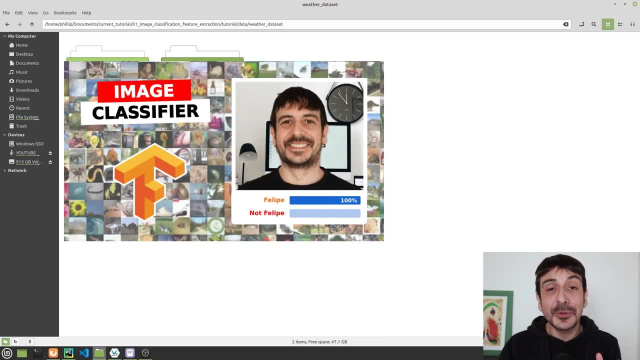 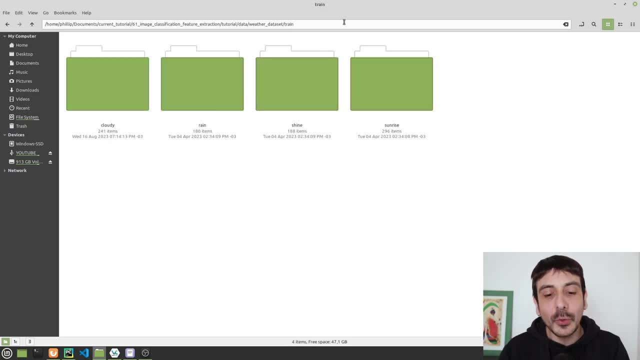 classifier using YOLOv8, and also in my previous video, where I show you how to train an image classifier using Teachable Machine. Exactly the same weather dataset. and now let me show you super quickly how this dataset looks like. You can see, we have four different categories. 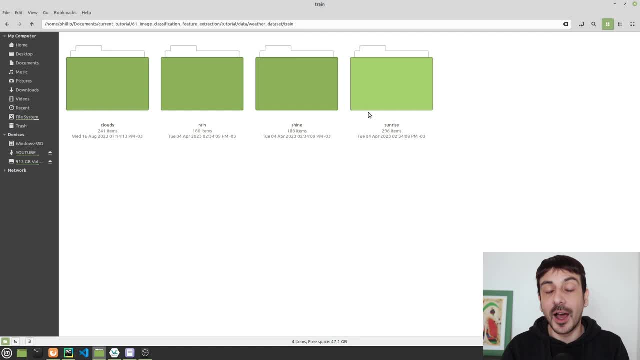 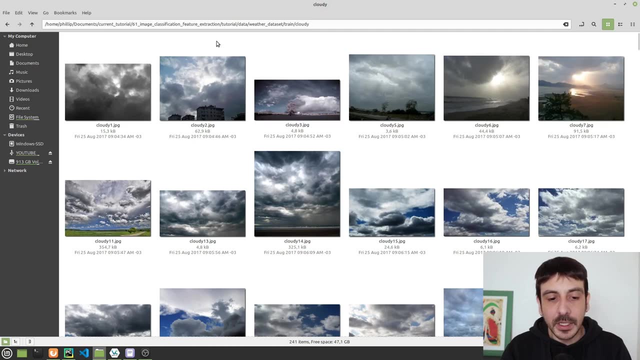 and these categories are cloudy, rain, shine and sunrise. Let me show you super quickly how each one of these categories looks like and you can see that this is the cloudy category. Now, if I show you the rain category, you can see we have many. 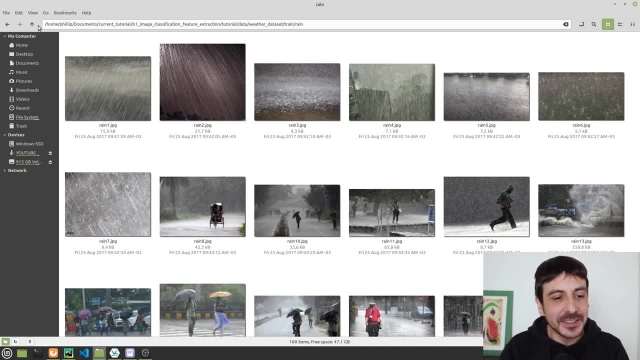 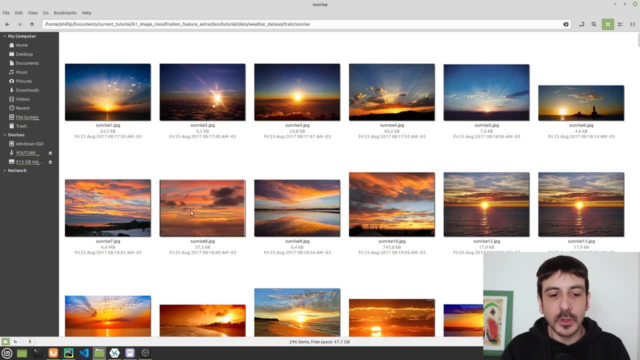 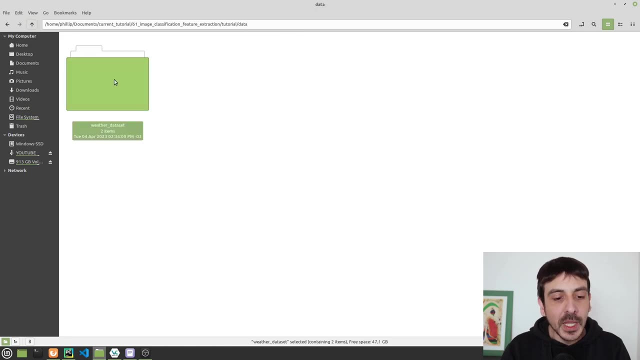 many, many pictures of super, super, super rainy days, and if I show you the shine category, this is how the images look like. and if I show you the sunrise category, you can see we have many, many, many pictures of sunrises. So this is the data we will be using in this tutorial and you can see we have 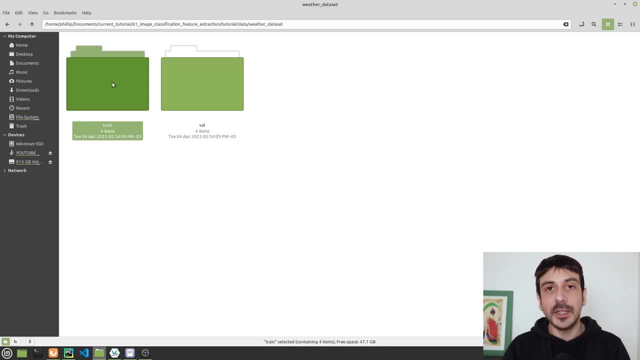 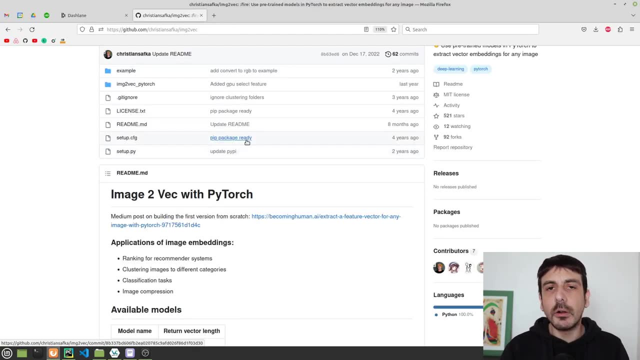 two directories. One of them is the weather dataset and the other one is the weather dataset is train, and this is where the training data is located. and then we have another directory which is called val, and this is the validation data. Now let me show you something else. If I go to 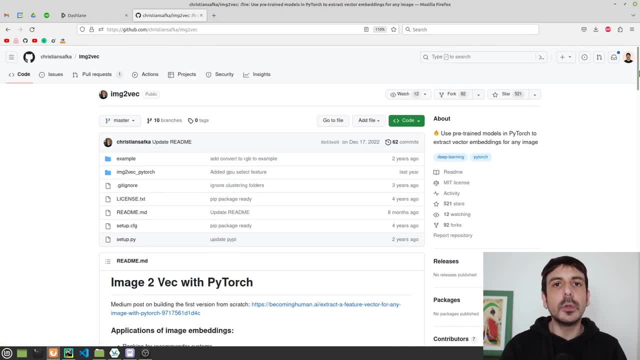 my browser. this is the github repository we are going to use as a feature extractor because, remember, in this tutorial we are going to work with image classification, but we're also going to work with feature extraction, and this is exactly how we are going to extract features from our images. This repository is called image2vec. 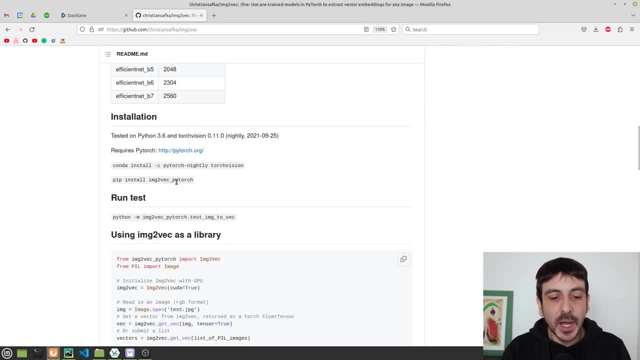 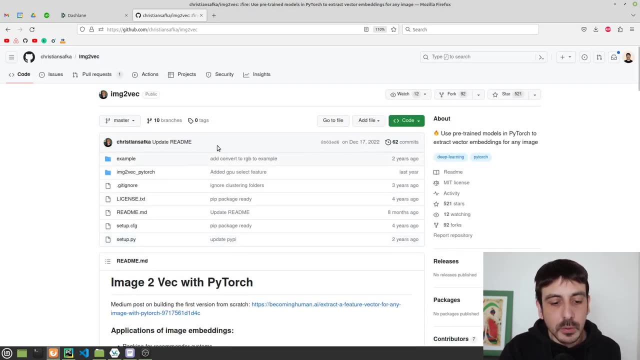 with pytorch, and this repository is available as a python package. so this is exactly how we are going to extract features from our images, and this is the repository we are going to be using in this tutorial. Now let's go to pycharm, because now it's time to start working on this tutorial. 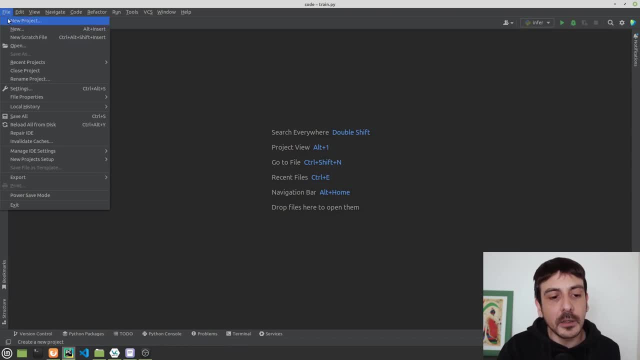 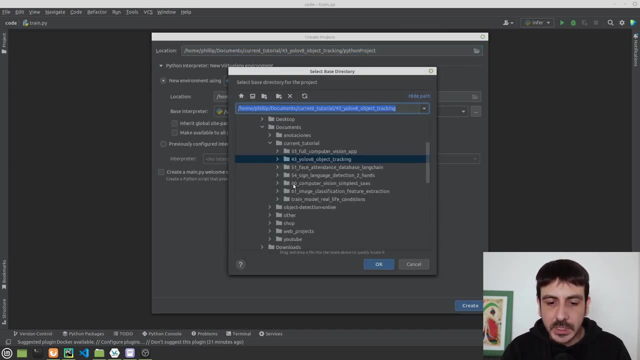 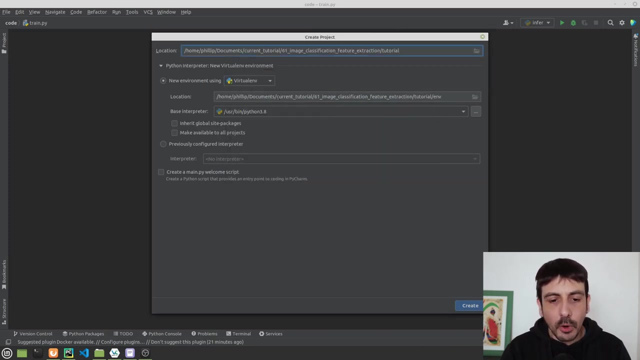 Now it's time to create a new pycharm project. so I go to file new project and I'm going to select the directory where I want to create this project, which in my case is something like here, tutorial. okay, and I'm going to create this new project using a virtual environment and python. 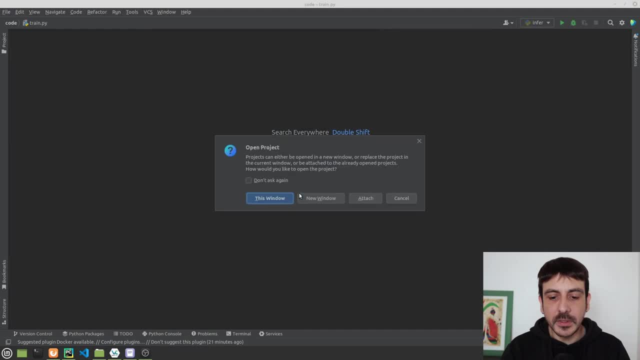 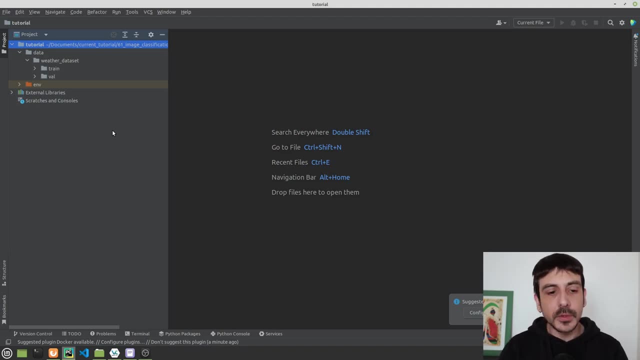 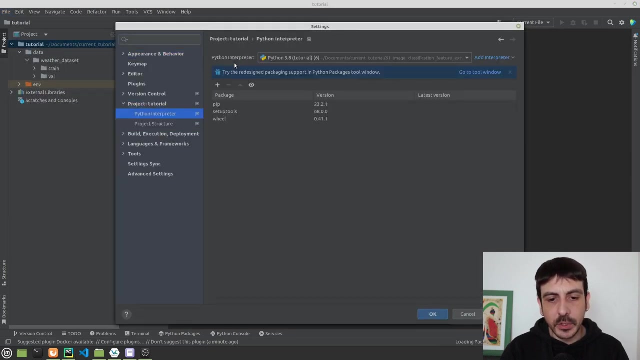 3.8.. I click on create. create from existing sources. this window, The pycharm project, has been created and now let's install the requirements we need in order to work on this tutorial. So I'm going to file settings, then project python interpreter. I'm going to click on this plus button. 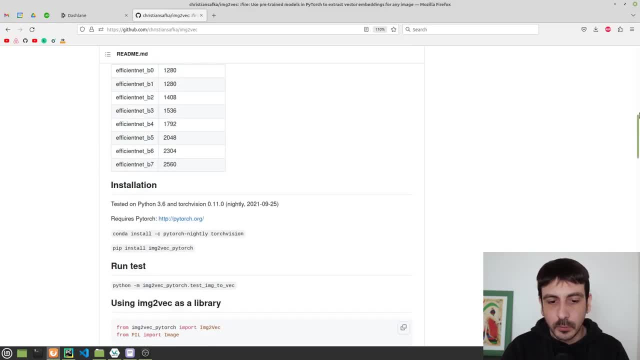 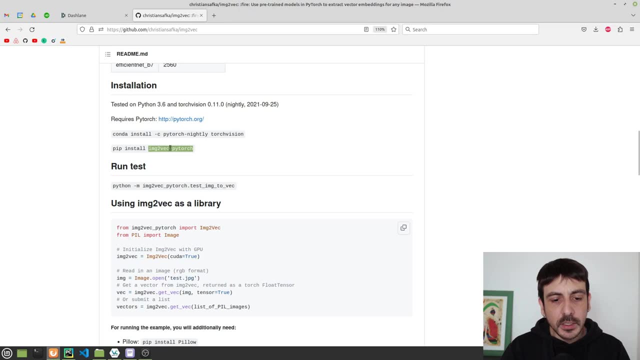 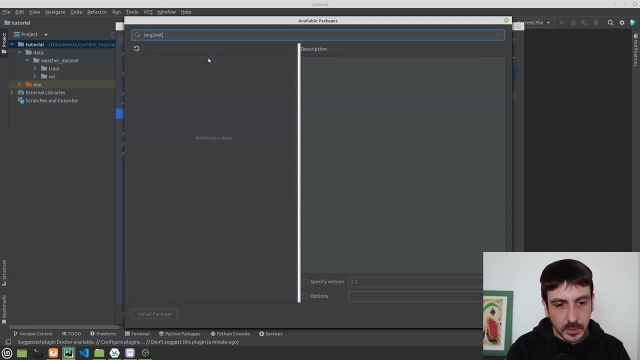 and the first library we are going to install is this one. right, we are going to work with this repository, so we are going to install this python package. so we need to install image2vec, slash pytorch. so let's find this library, image2vec, and this is 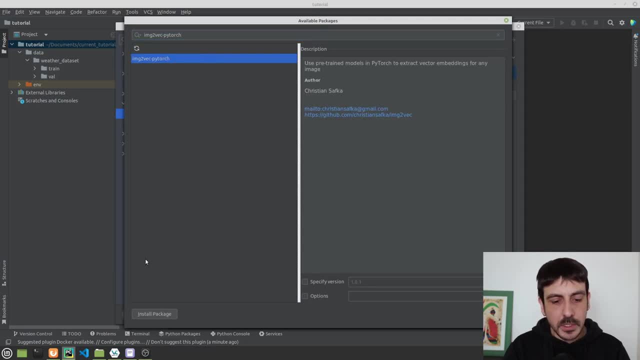 the one we need by torch. okay, I'm going to click here and then install package, and that's pretty much all. then we also need to install two additional libraries. one of them is seekitlearn. so I'm going to search for seekitlearn, this one, over here. I'm going to press install package. 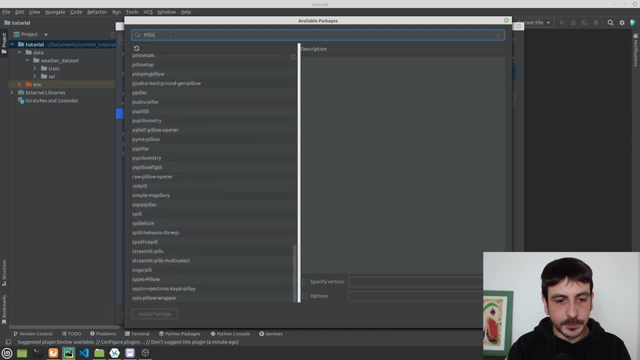 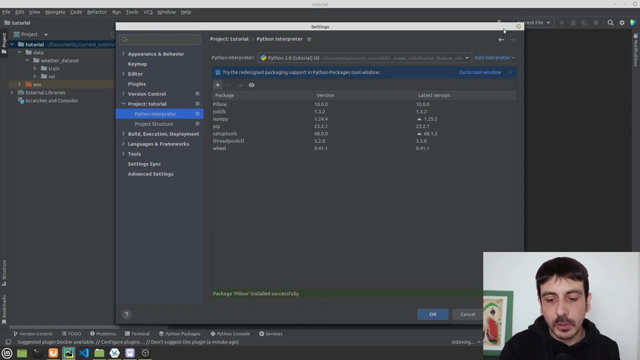 and then I also need to install pillow, and that's pretty much all. so my python packages are being installed, but in the meanwhile, let's start working in this tutorial, let's start working on all the coding of all of these tutorials. so I'm going to press here on, ok, and then I am going to create a new file, which is mainpi. 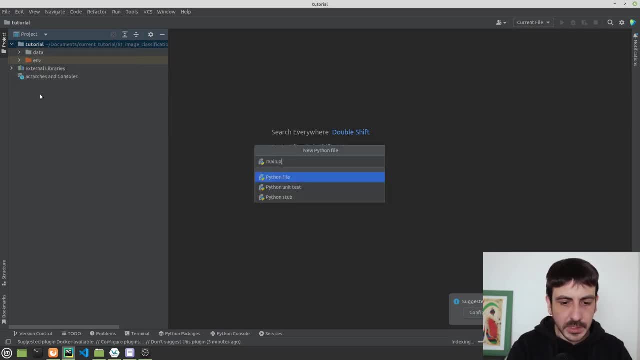 mainpi. okay, and this is the file we are going to use in order to train our image classifier, in order to do the feature extraction and also the image classification. so I am going to enlarge it a little and the first thing I'm going to do is to write the four steps we will take in order to 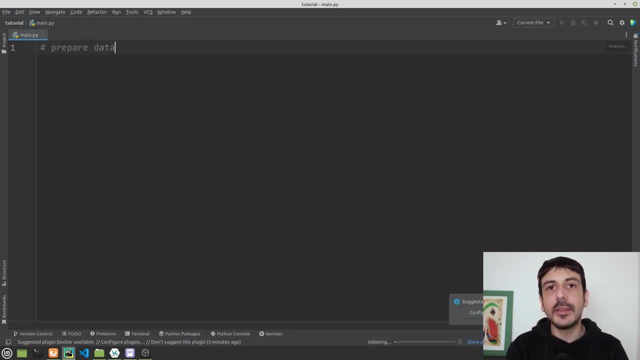 complete this process. the first one is to prepare the data we are going to use in order to train this classifier. then we are going to train our image classifier and then we are going to train the model. we are going to train a classifier, then we are going to test the performance of this. 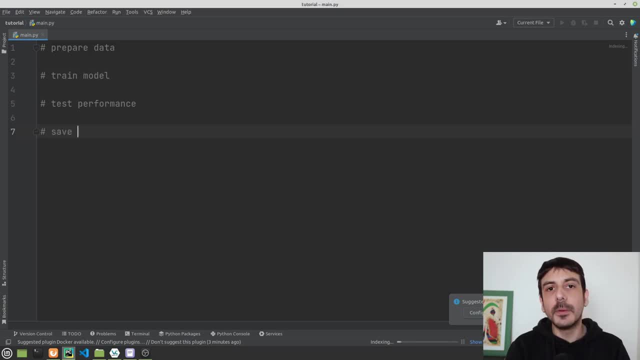 classifier. and, finally, we are going to save the model into our computer, right? so these are the four steps of today's tutorial, and now let's get started. and the first thing we need to do is to import from image to back. pytorch import image to back. okay, and then we are going to create. 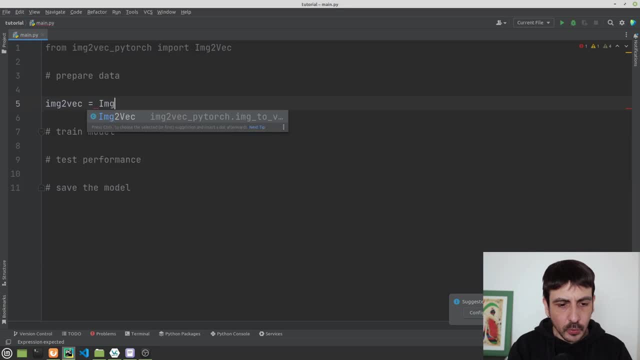 image to back. we are going to create a new object which will be the feature extractor we are going to use in order to extract features from our images. and now let's prepare the data. so I am going to define a new variable which is data directory, and this is the directory. 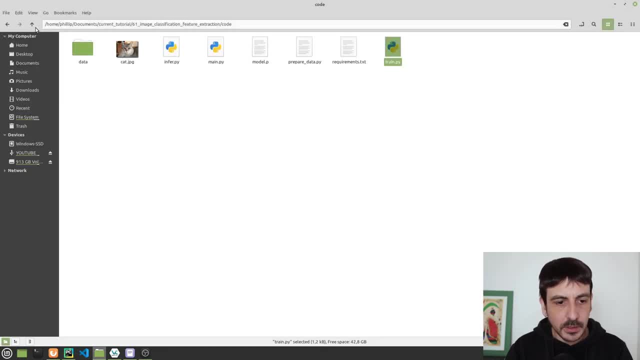 where my data is located, and my data is located in the current directory. this is directory where I have created this project. this is the mainpi file in which we are currently working in, and this is where my data is located. it's in a directory which is called data, and. 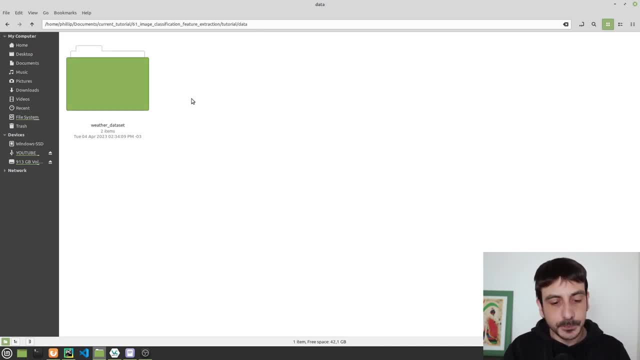 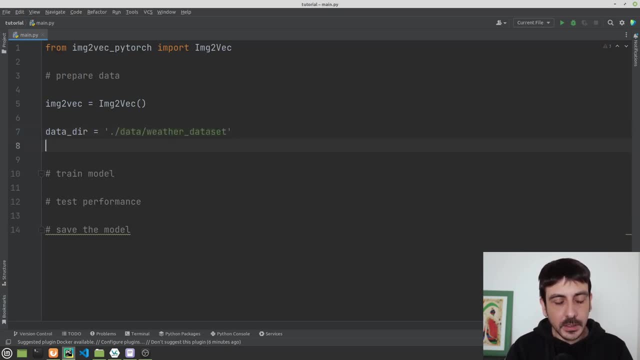 within this directory, there's another directory which is called weather dataset, so i am going to define the data there as data weather dataset. then let's create two additional variables. one of them will be train directory, and this is where my training data is located, which is here. 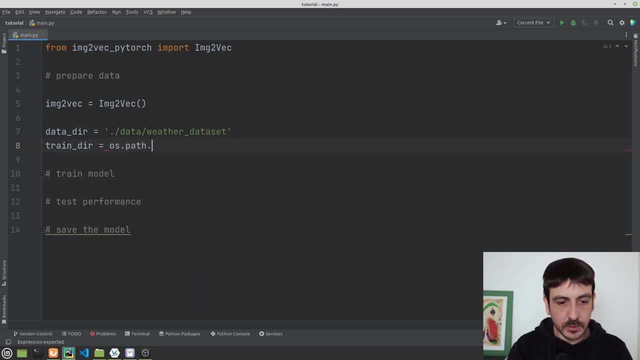 let's do something more like this: ospat, join data directory and then train- okay, and then the validation directory, which is going to be something like this: okay, and i need to import os, otherwise this is not going to work. so import os, okay, and that's pretty much all remember. within weather dataset, we have two directories, one of 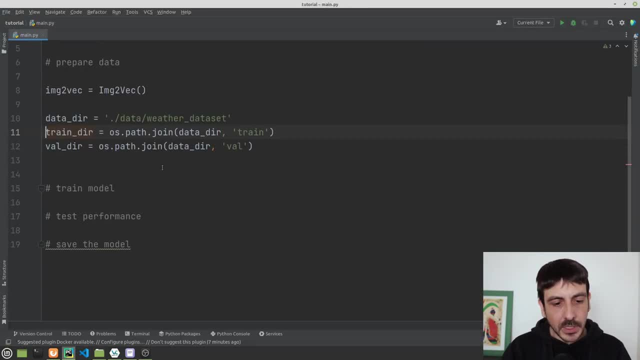 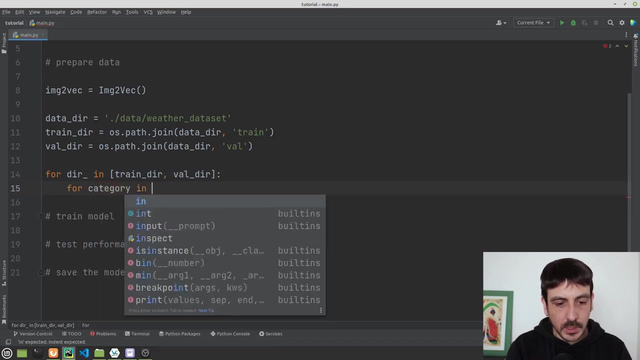 them is called train and the other one is called val. now let's continue. now let's walk through all the files in these two directories and this is how we're going to do: for dir in train directory, val directory for caten category in os list: dir. 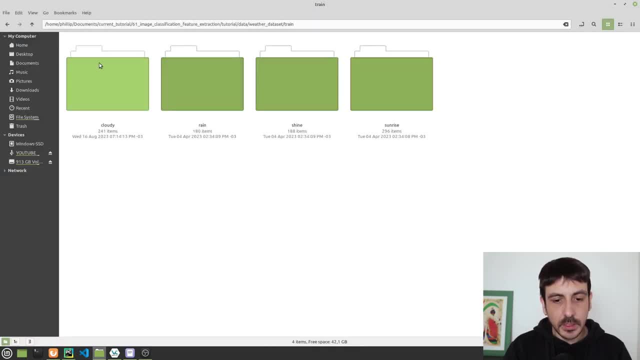 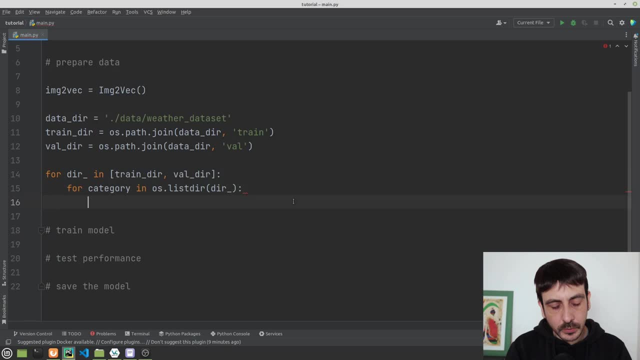 directory. right, we are going to iterate in each one of these categories and we are going to define another variable. we're going to make another loop which will be for image path. in us, let's do os path join dir category, right, so we are iterating in all the images which are within this directory. right? so we are. 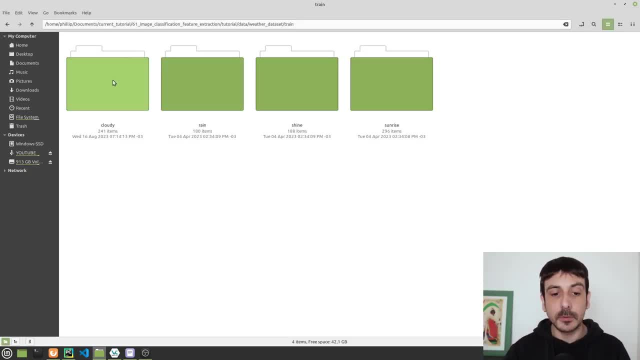 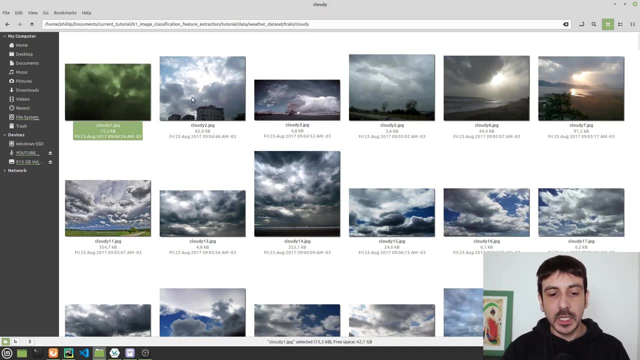 iterating in all the categories. so we are iterating in each one of these four directories you have over here and then, for each one of this directory, we are going to iterate in all the images you can see over here right now. we are going to define another variable, which is going to be image. 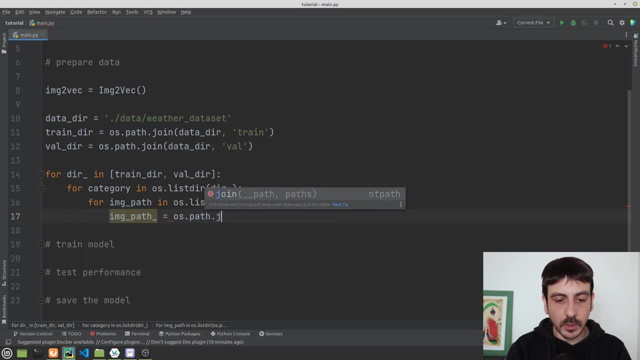 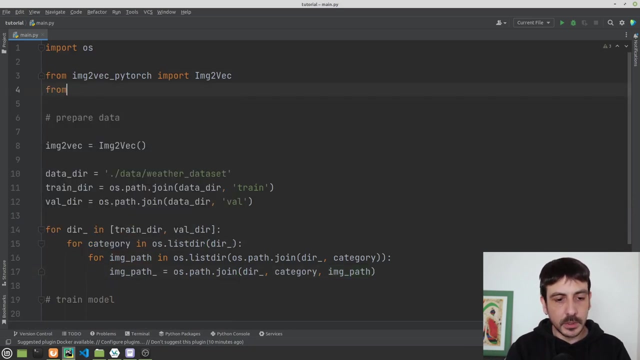 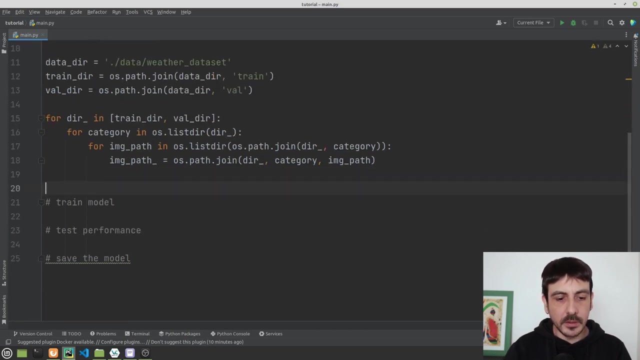 path underscore. and this is os part. join directory category and then image parts. okay, then we are going to make another import, which is from peel import image, because we are going to read each one of these images, we are going to load each one of these images like this: imageos. 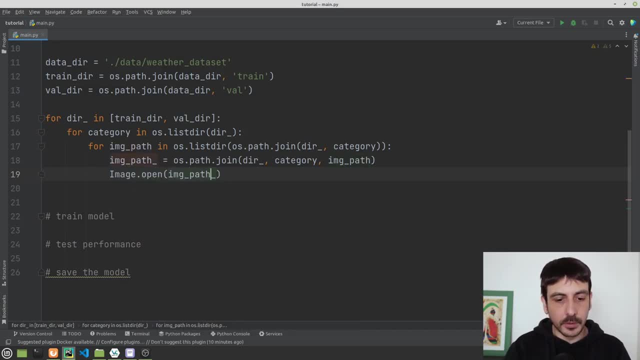 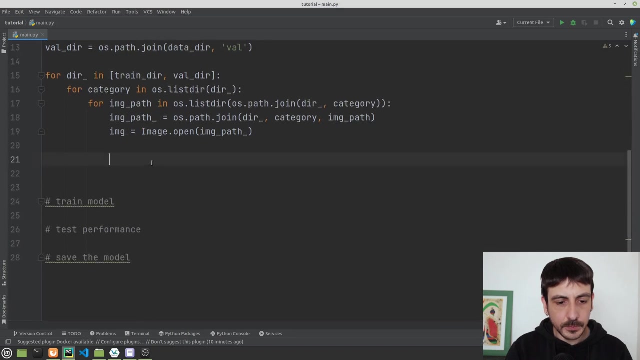 open image, part underscore, and this will be image. okay, and now we are going to compute all the features from this image and this is how we're going to do: we are going to call image to back, dot get back, and we are going to input the image and that's it. this is all it takes. 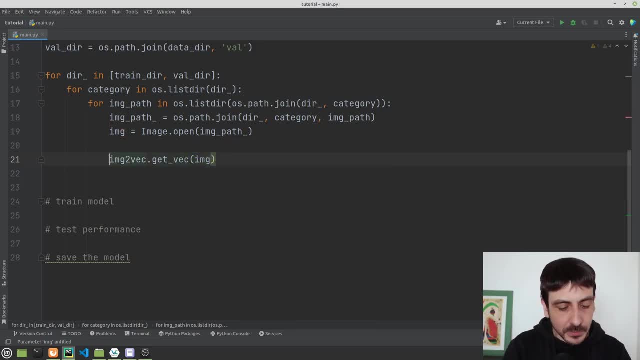 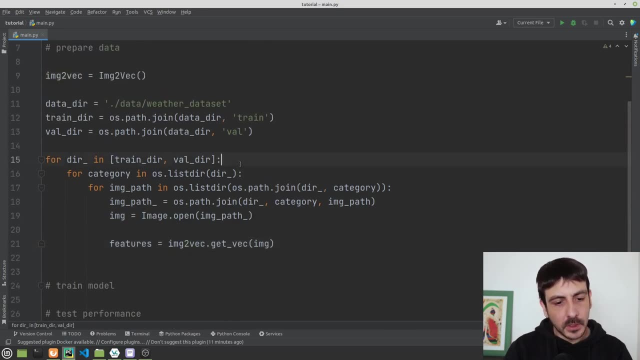 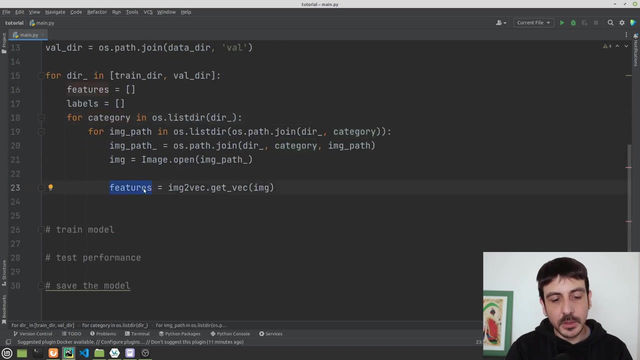 to compute all the features from this image and this is going to be something like feature features. okay, now i am going to create two lists. i'm going to do it over here. one of them will be features and the other one will be labels. okay, and this object- maybe it's a 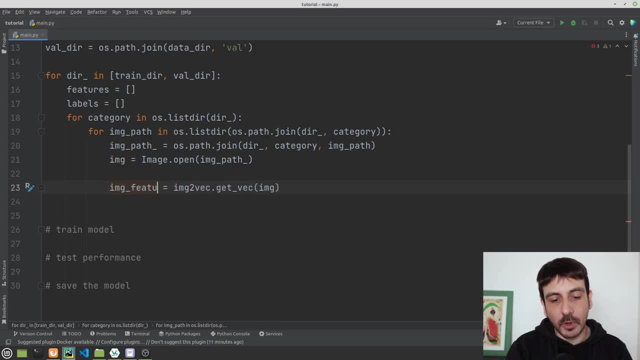 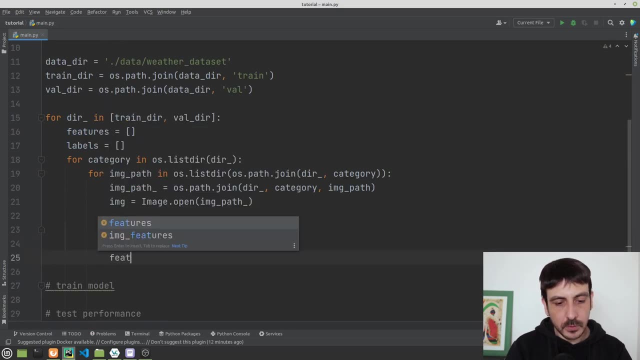 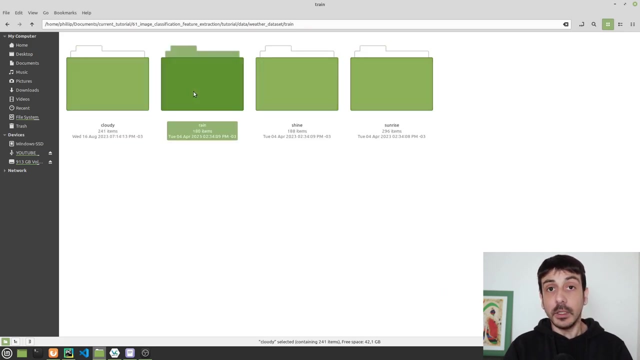 better idea to call it something like image features, right, something like that. and now we are going to append featuresappend- image features right- and then labelsappend, and the label will be something like the category- right, these are all labels. the each one of these directory names is all categories, right? these are all. 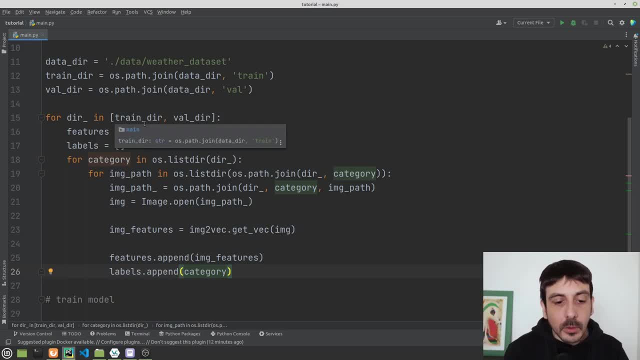 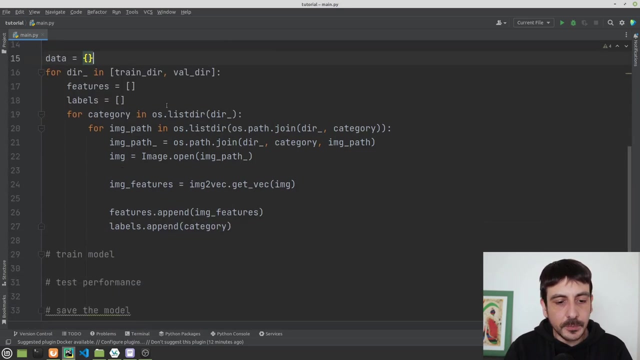 four categories. so, in order to append the label, we need to append the directory name, we need to append this variable over here, which is called category. now let's continue. now i'm going to define another variable, which is data. this is going to be a dictionary and i'm going to do 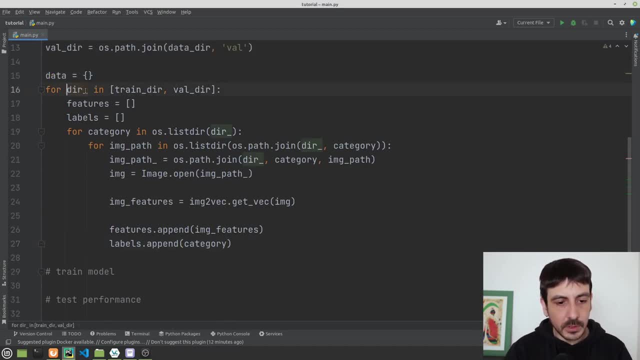 something like this. i am going to walk not only in the directories, but i'm also going to define another variable, which is going to be jdir, in enumerate train, dir, baldir, something like this. so now this is going to take these two values dear is going to be trained here in the first. 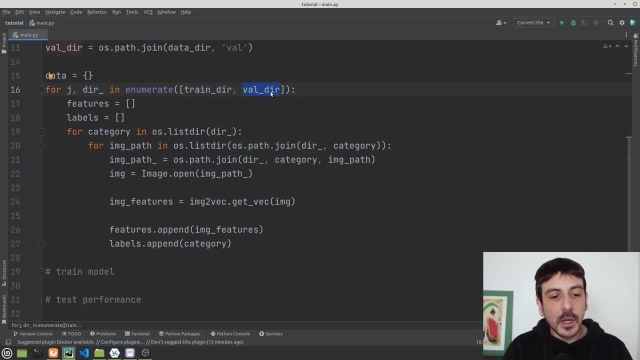 iteration, and it's going to be baldir in the second iteration and j will be zero in the first iteration and it will be one in the second iteration. so by doing so, we can do something like this. now i'm going to say data training, data validation, data. 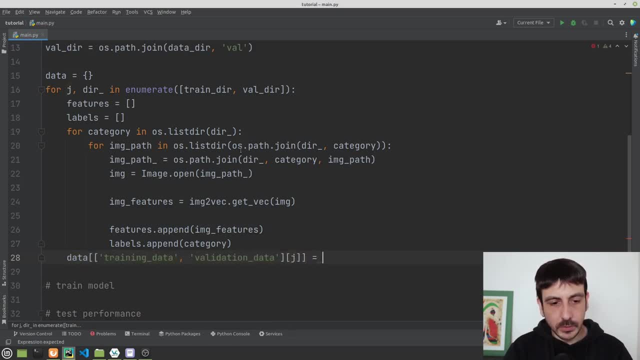 and this will be j, equal to features, and then the same, but with the labels: training labels, validation labels, j and this will be labels, right? remember that in the first iteration there is training directory and j will be zero. so if we access the index number zero from this list, we are going to get training data and then in the 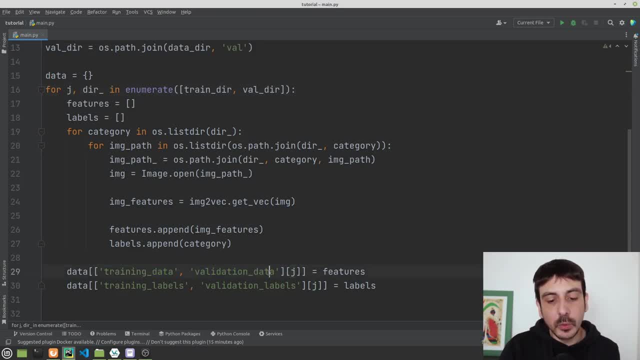 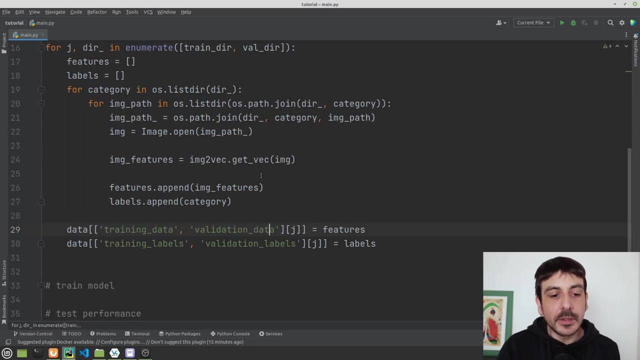 second iteration, j will be one. so we we are going to access the second element, which is validation data. so we are going to create this key according to the iteration we are in, and the same is going to happen for the labels, right? but in order to be more clear, let me show you exactly how this 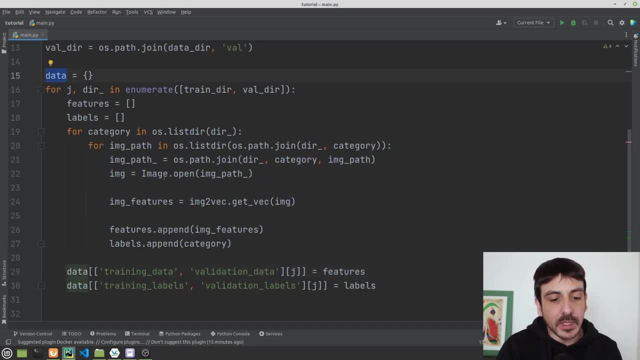 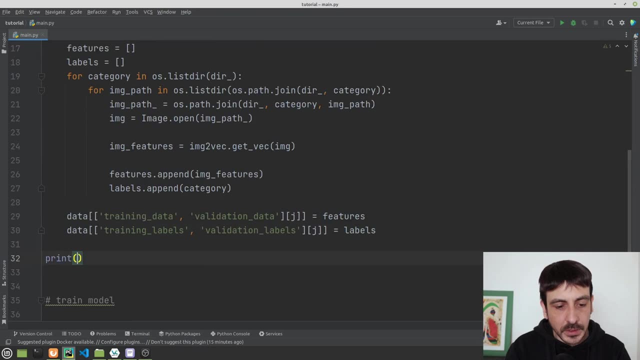 variable we have over here, how this dictionary we have over here, how it looks like. so i'm just going to execute the code as it is and at the end i'm going to say something like print data dot keys. right, let's take a look at this dictionary we have over here and let's see. 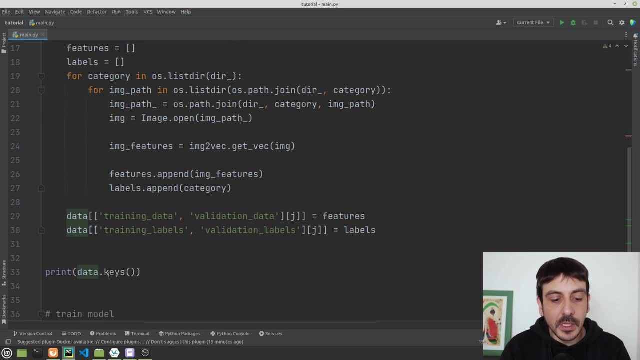 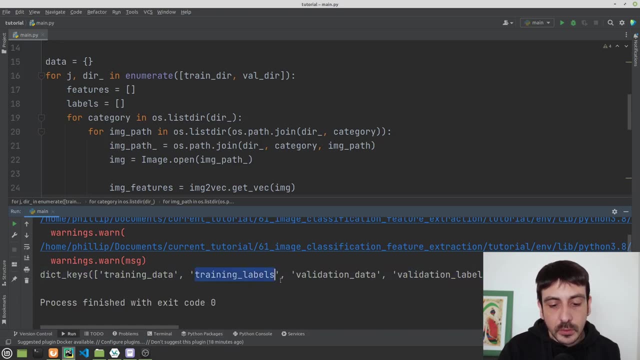 exactly how it looks like. let's see exactly what are the keys for this dictionary, so i'm just going to press play. okay, the execution is now completed and these are the keys we have saved in this dictionary: training, data, training labels, validation- data- validation labels. so i'm 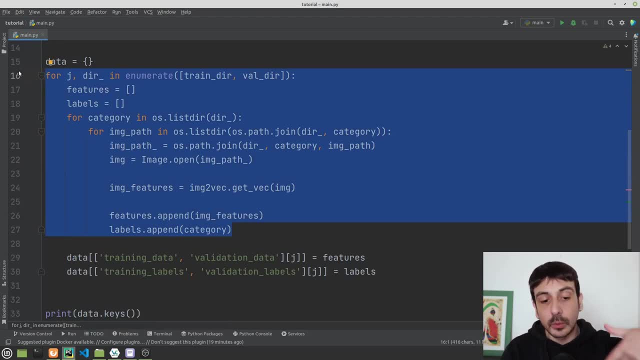 i invite you to take a look at this code. i invite you to to go through this code once and again until it's 100 clear for you exactly what we are doing over here. please notice: we are iterating in all the images, in all the training images and all the validation images. we are 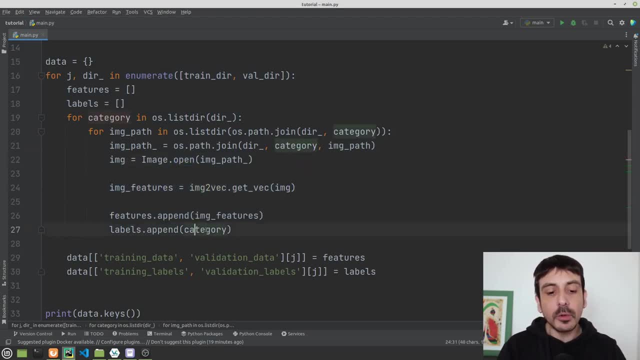 opening these images, we are computing the features, and then we are saving this data into these two lists we have over here, and then we are saving these lists in this dictionary under the very appropriate keys, right? so please go through this code once and again until it's 100. 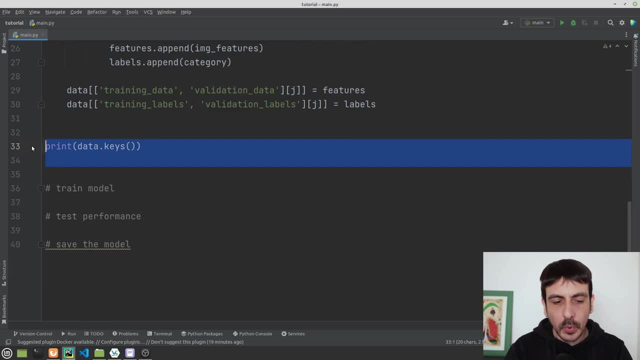 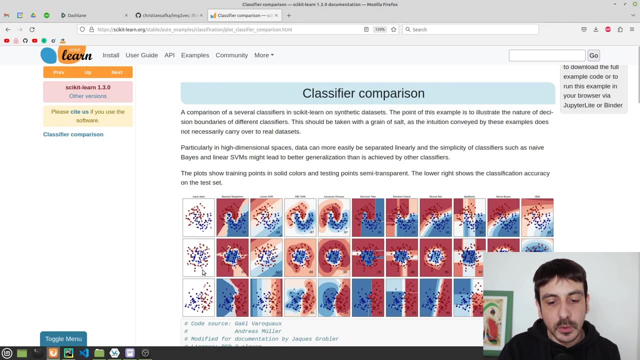 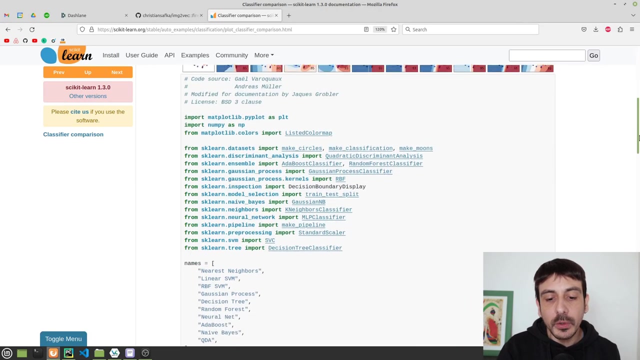 clear for you, but for now, let's continue. we have saved all of our data into this dictionary and now it's time to train the model. in order to train this model, let's go to my browser super quickly, because we are going to use a model, a classifier from ckit learn and let me show you all the 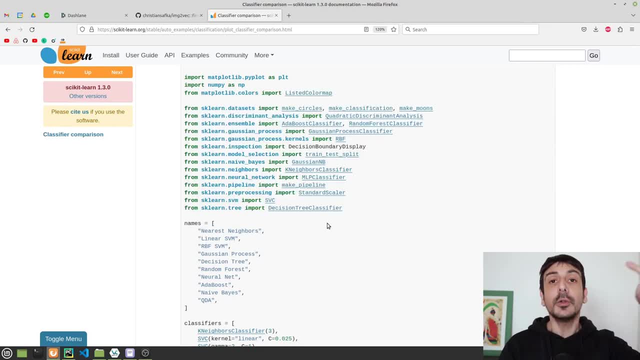 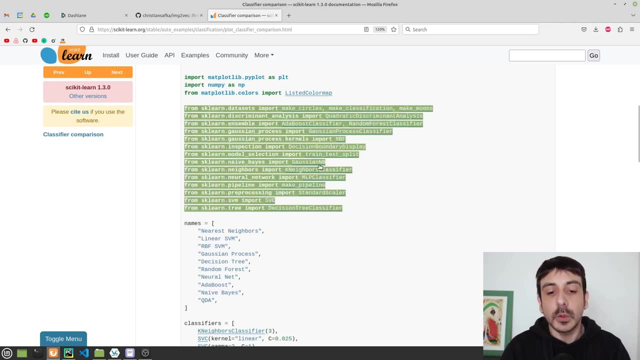 different classifiers we could use from the secret learn. i also invite you to take a very close look at this website so you are more familiar with all the different classifiers you could use from ckit learn. in this tutorial, we are going to use random forest classifier. we are going to use this. 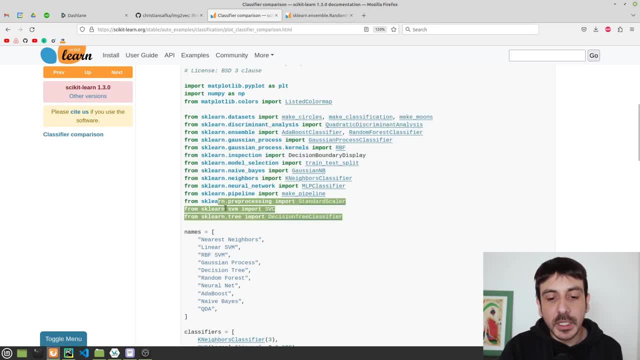 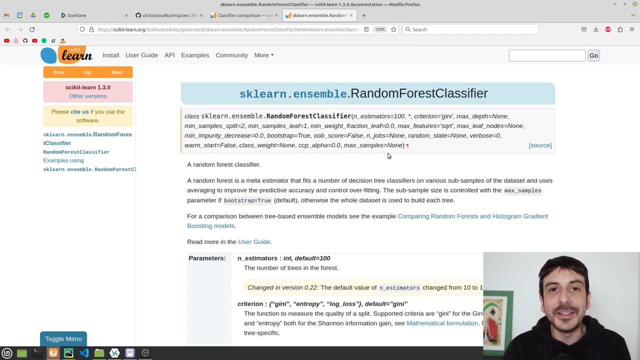 classifier over here, but we could also use any other classifier from here, right? the only reason we are going to use a random forest classifier is because i like it. i really like this classifier. i have used it many times in many projects. i think it's very robust, it's very easy to use. it's very 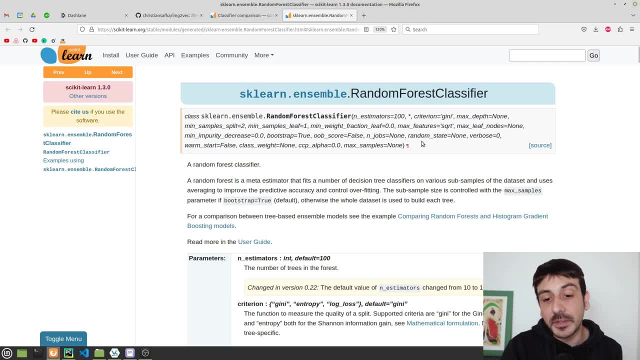 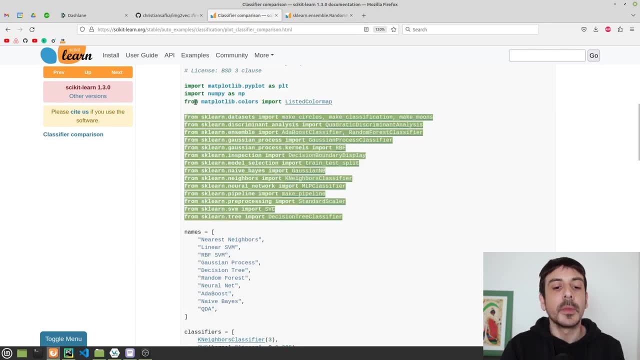 easy to understand what's going on. i really like this classifier, but that's the only reason why we are going to use a random forest classifier. we could also use any other classifier from here. so let's go back to python. and now i'm going to make another import, which is: 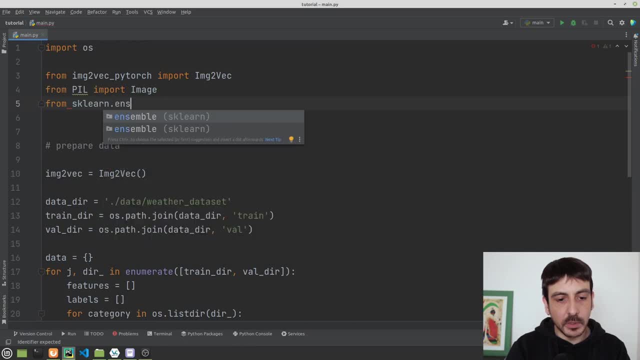 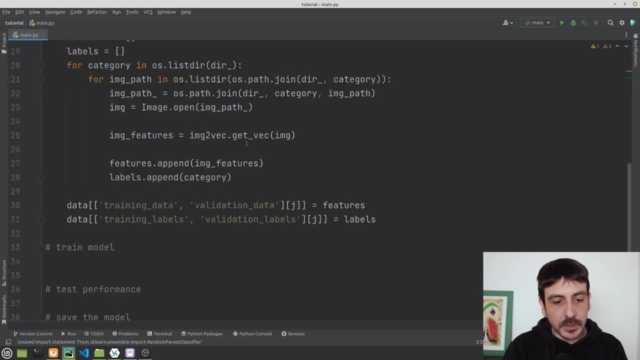 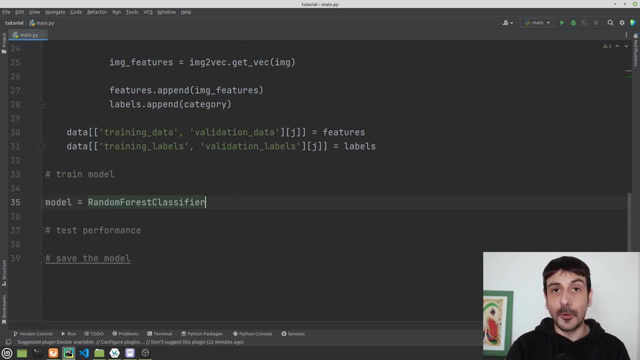 from sklearn dot ensemble import random forest classifier. and then i am going to take this value- random forest classifier- and i'm going to define a new. another variable is called model and model will be random forest classifier. right, we are creating a new instance of this classifier and then, in order to train the model, the only thing we need to do is to call. 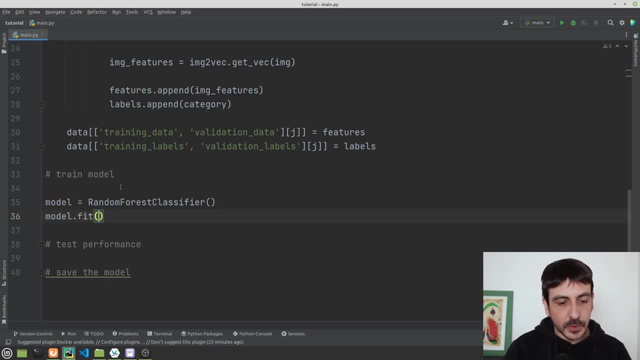 modelfit. we need to input the training data, which is here, the training labels, which are here, and that's it. that's all. that's all it takes in order to train this classifier. you can see how simple this is now. let's continue. now it's time to test the performance of the image. 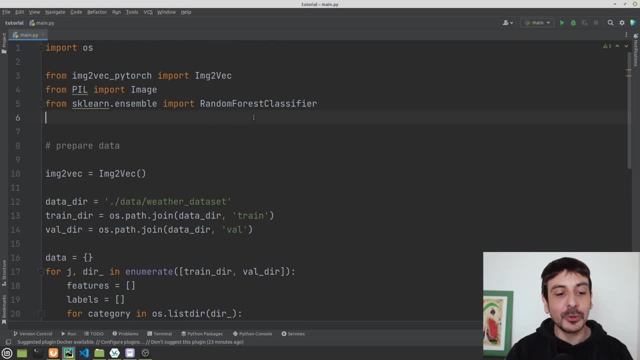 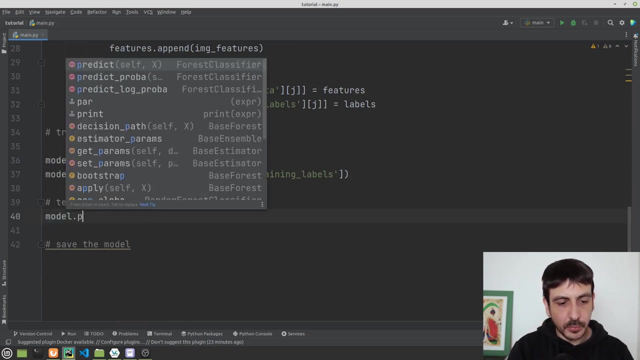 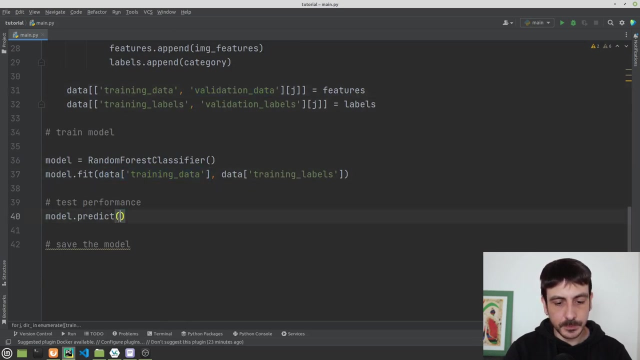 classifier we have just trained in order to do so. i am going to make another import, which is from sklearn dot matrix import accuracy score, and i'm going to make something like this: modelpredict validation data. sorry, data validation data. we want to access our validation data, which is saved. 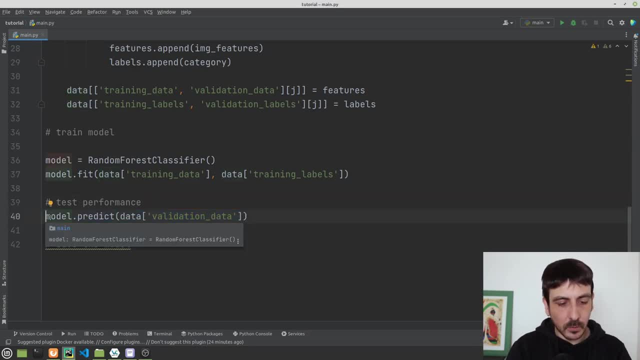 here and this will be something like y pred. then we are going to call accuracy score, we're going to import, we're going to input y pred and we're also going to input data validation labels. okay, so you can see, we are computing the accuracy score with the validation data, which is completely and absolutely unseen data for our model, for our 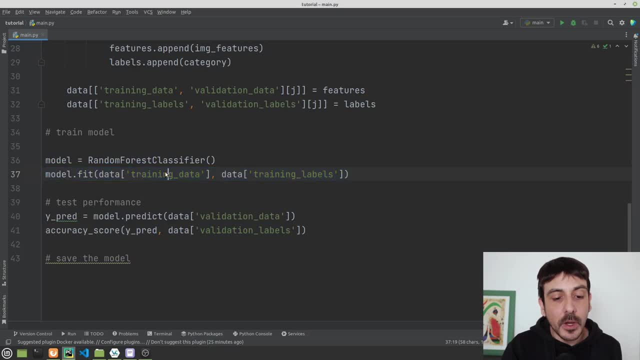 classifier. you can see here we are training our classifier with the training data. the validation data is completely unseen data. the classifier has never seen this data before. so this is exactly the type of data we should use in order to compute the accuracy score, in order to test the performance of our model. so this is going to be something like score. 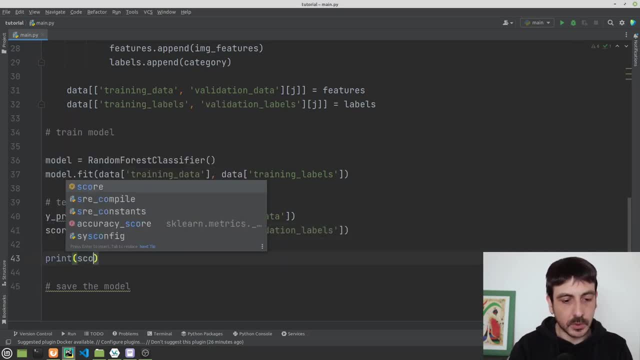 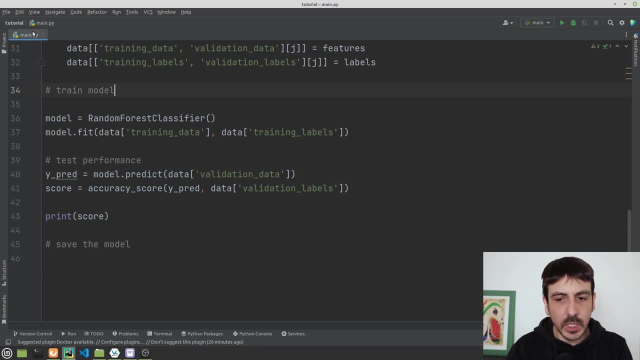 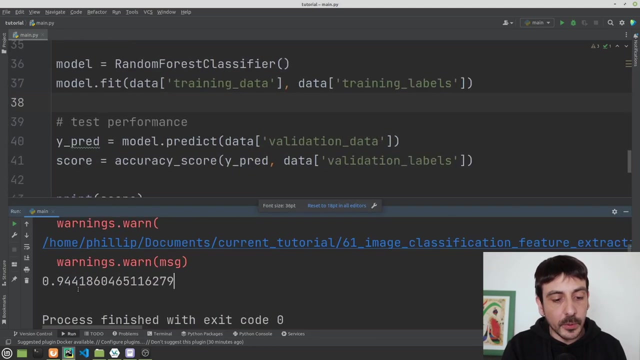 and now i am going to print score instantly. we are going to say the model, but let's take it one step at a time. let's execute this script, let's see its everything. if everything is okay, okay, the execution is now completed. we didn't have any error whatsoever. 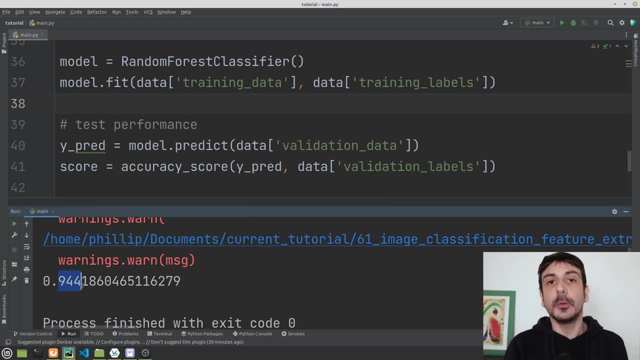 and this is the accuracy. we had a 94.4 accuracy, which is a very, very, very high level of accuracy. now, remember i told you this is exactly the same data set we used in two of my previous videos: in my previous video, where i showed you map and vector code. the next example is data arrangement. 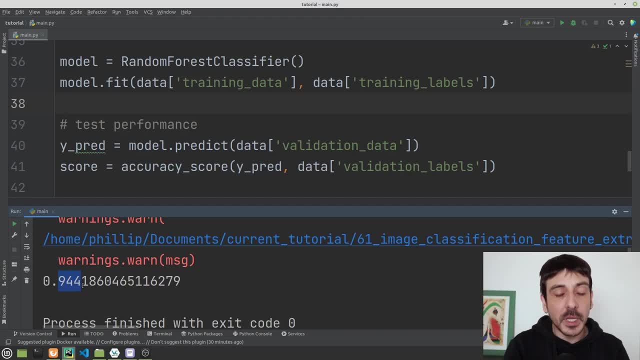 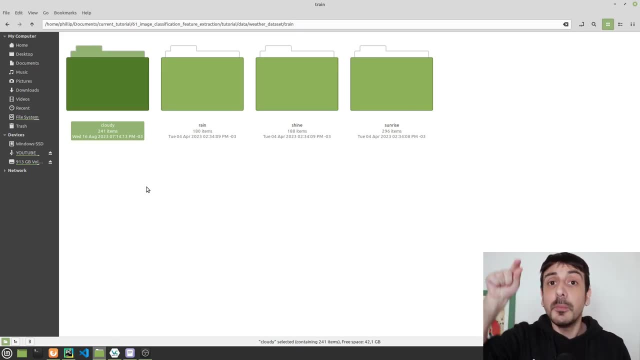 you how to train an image classifier using yolo v8, and also my previous video where i show you how to train an image classifier using teachable machine. this is exactly the same data set, so i invite you to take a look at those two videos and to compare the accuracy we are getting here. 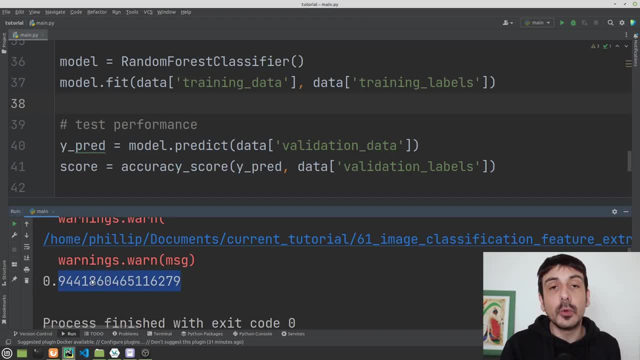 with this classifier, with the accuracy we got in those two videos right, using yolo v8 and using teachable machine. i invite you to compare this accuracy with the accuracy we got in those two other videos. that's your homework. that's your homework from today's tutorial. and now let's. 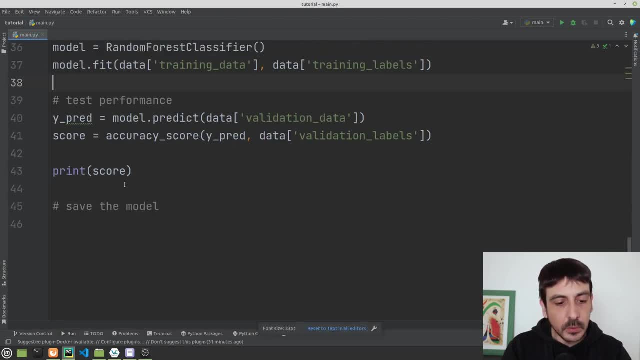 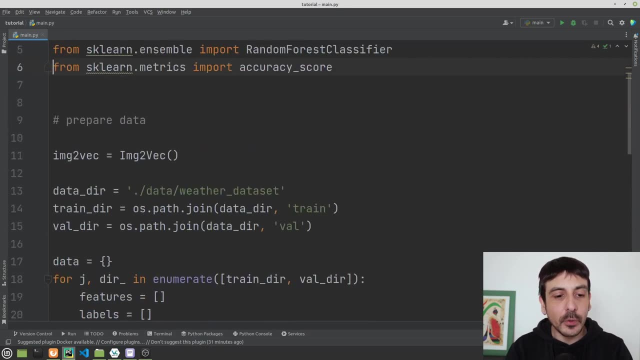 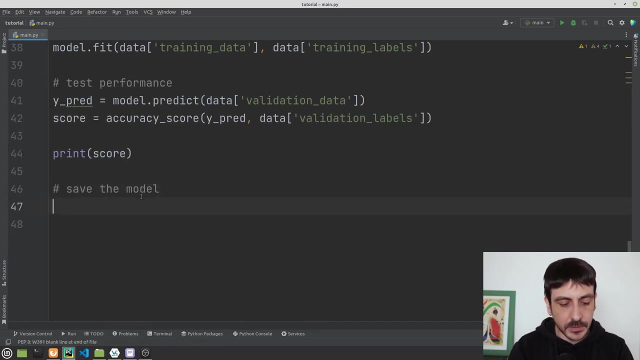 continue. so the only thing we need to do now is to continue to the next step, which is saving the model, and this is how we are going to save the model. we are going to import another library, which is pickle, and we are going to say something like this: with open the name, the file name will be: 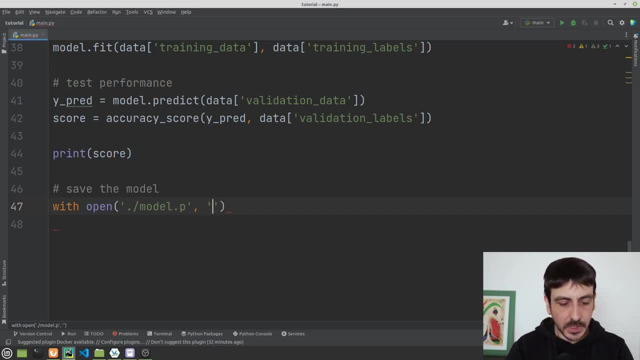 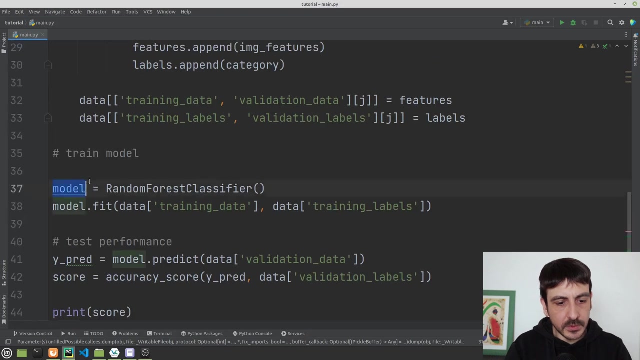 something like modelp. this will be wb as f and we are going to call pickledump. then this will be the object we are going to save, which in our case is model, and then f, and that's pretty much all. then i'm going to close the file. 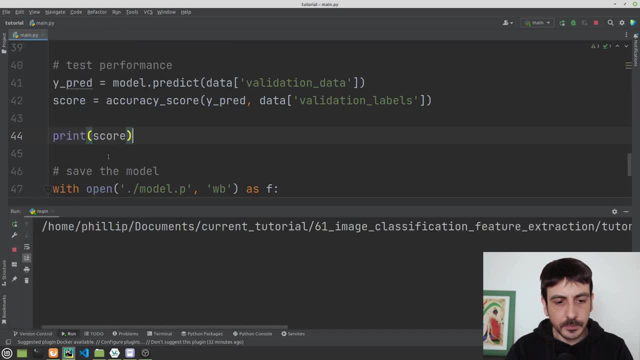 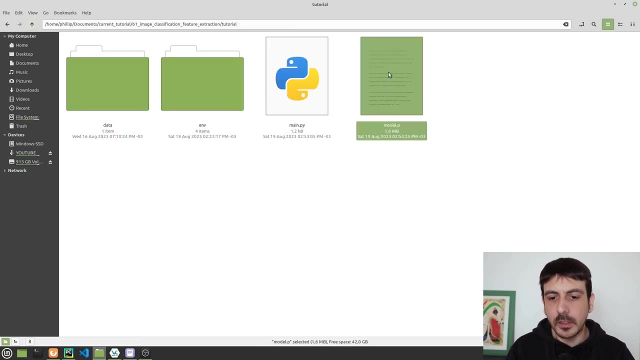 and now i'm going to run this file again. okay, and now, if we go to my file system, you can see that now we will have a file which is called modelp, and this is the model we have just saved. so everything is working just fine. and now let me show you how to take this model, how to load this. 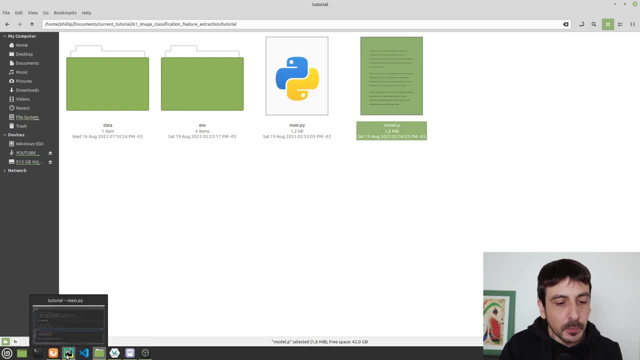 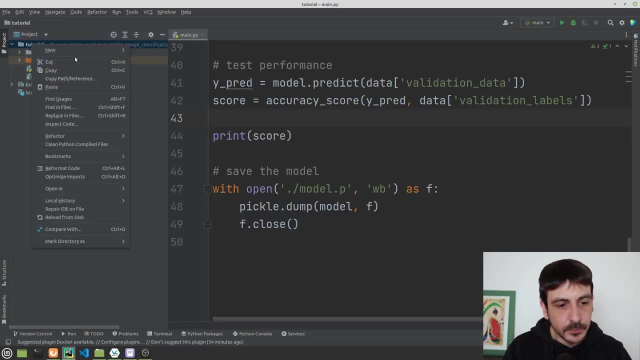 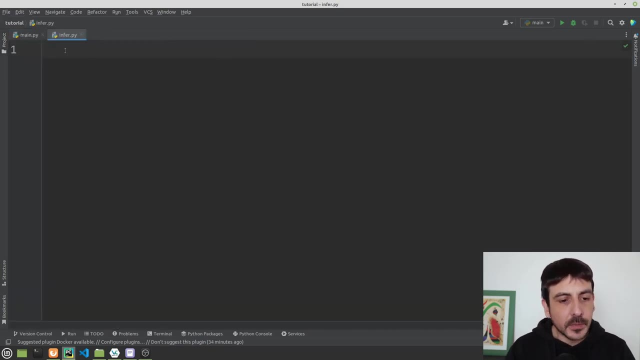 model to produce inferences with it, right? so i'm going back to pyjarm and i'm going to create a new file which is called inferpi, and this is where we are going to make our inference. so i am going to take a few lines from here. i am going to import this object and i'm also going to 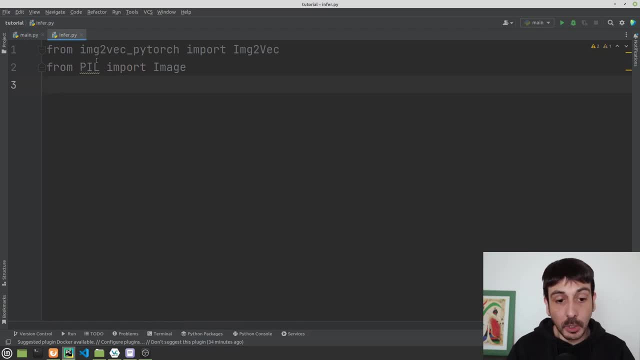 import this other um object from peel, and then this is going to be a very, very similar process. i'm going to create this object over here, which is image2vec. this is the object we are going to use in order to compute our features, and then i'm just going to define an image path which will be 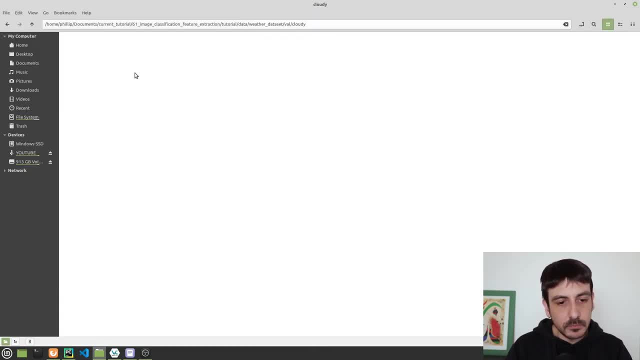 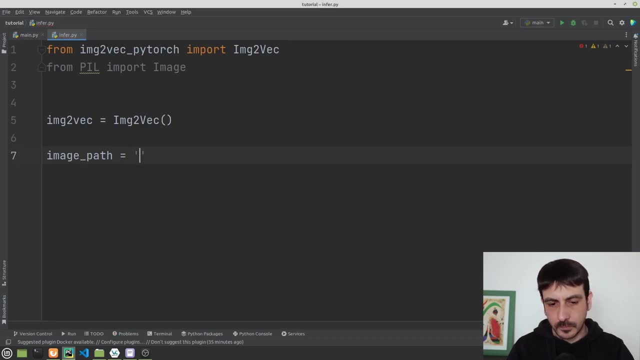 one of my images in the validation data. i'm just going to take a random image, something like this: claudy4.jpg, a random image in this directory, and then i am going to do something like. image will be imageopen- image path, and then i am going to. 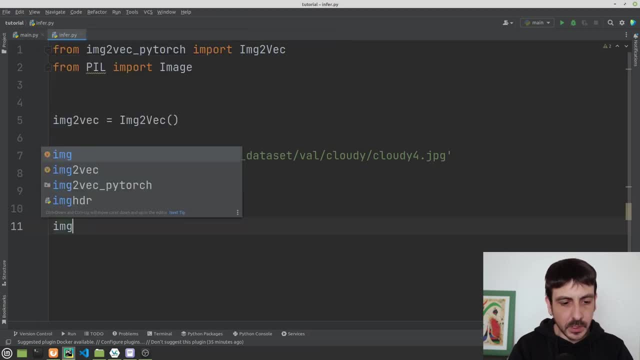 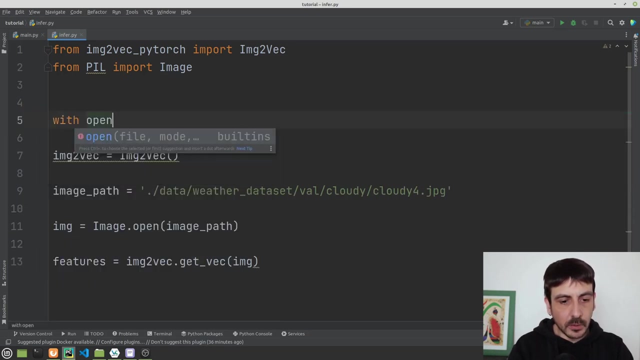 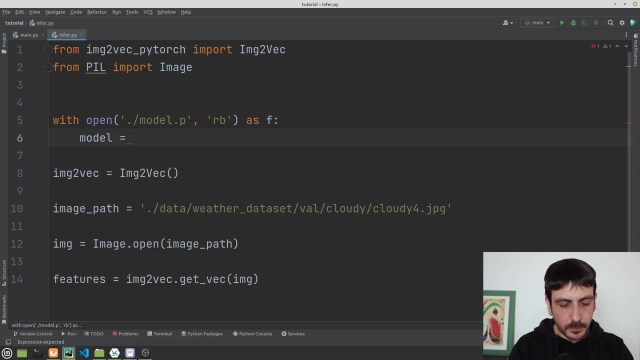 compute features from this image, doing something like image to back, image to back dots, get back image. this will be features. ok, then I am going to load the model, or maybe I can load the model over here. so I'm going to say something like: with open model p, this will be our B ask if and model will be pickle dots. 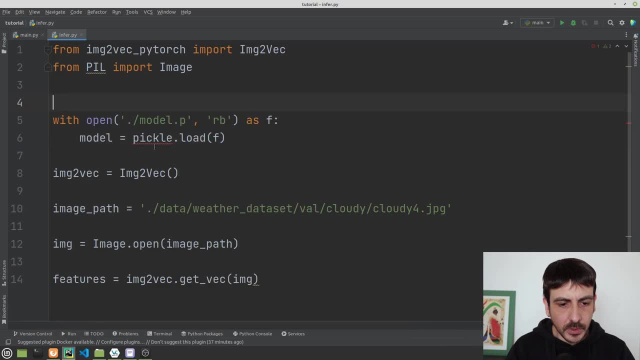 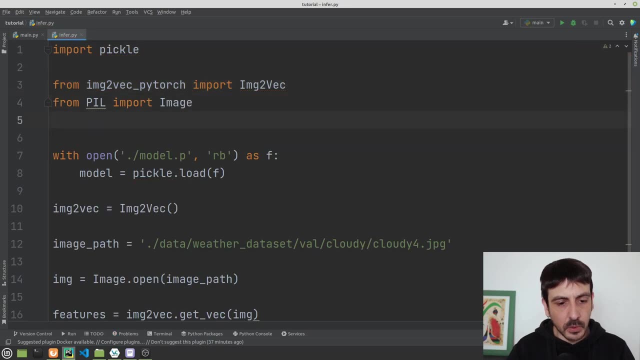 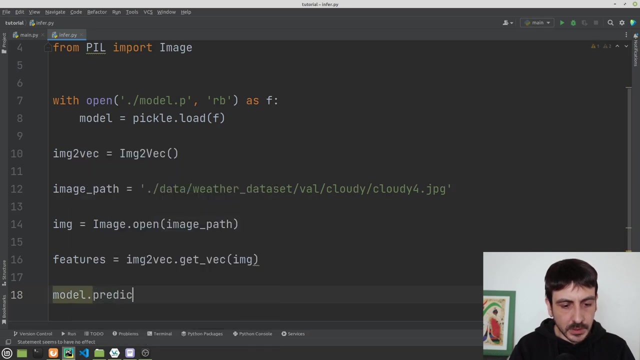 low will. if- and obviously we need to import pickle, or is. this is not going to work. import pickle, and that's pretty much all. and now we are going to call model dot, predict, and we are going to input the features, and this is how we are going to do it.